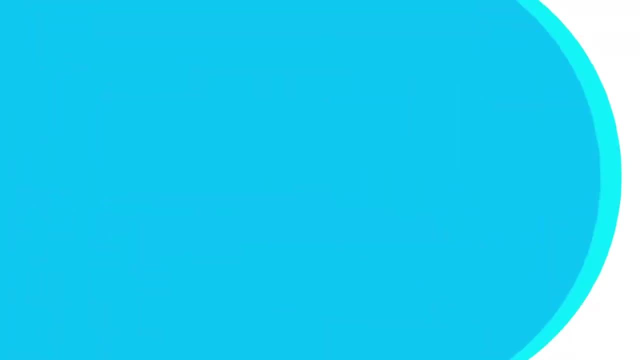 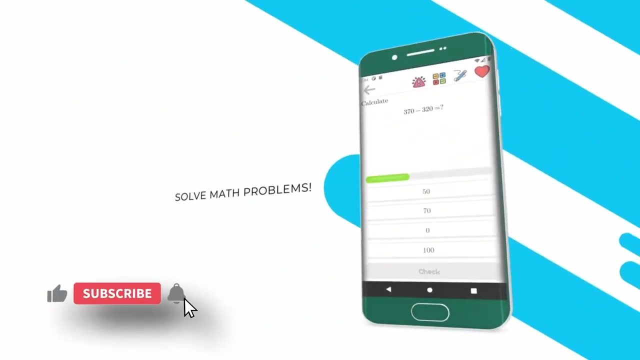 if you are a university student or you are in a grade one to eight, the app can help you with math learning and solving math problems. the application will help you master basic math in a short time. if you are an adult, you can train your brain and solve. 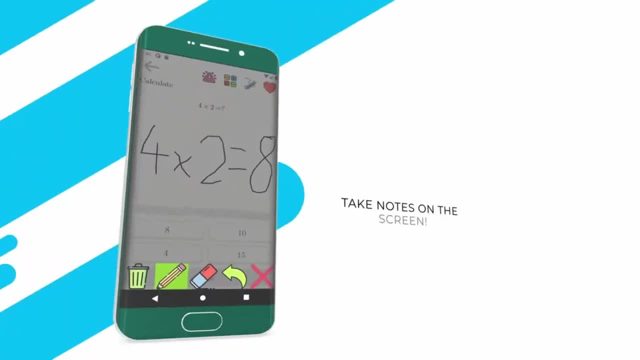 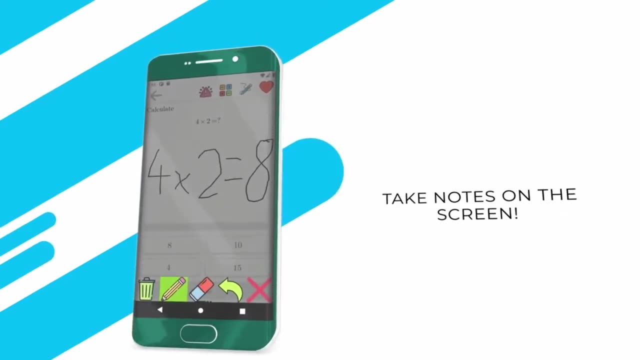 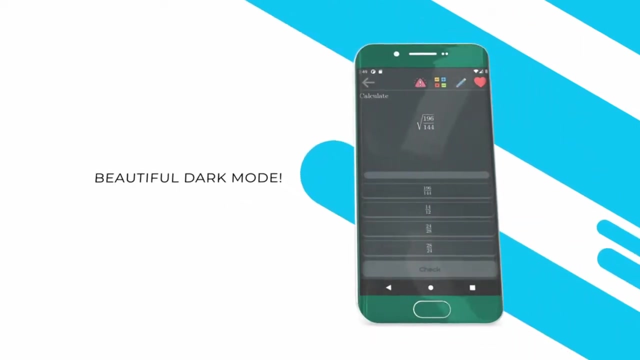 each task has an answer that explains the solution step by step. the app helps children get into habit of learning and practicing math every day. be active and exercise math problems to get interesting rewards, unpoints and unlock new levels and ranks the preparation for the test and exam at school. 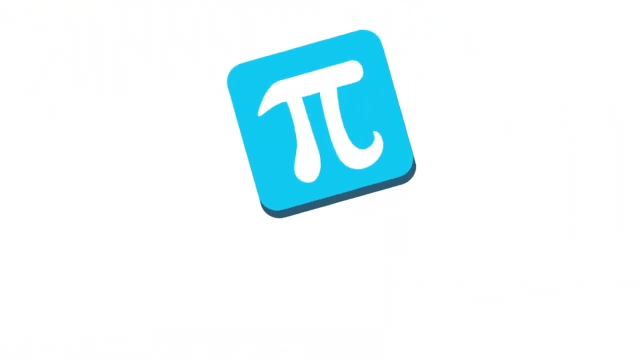 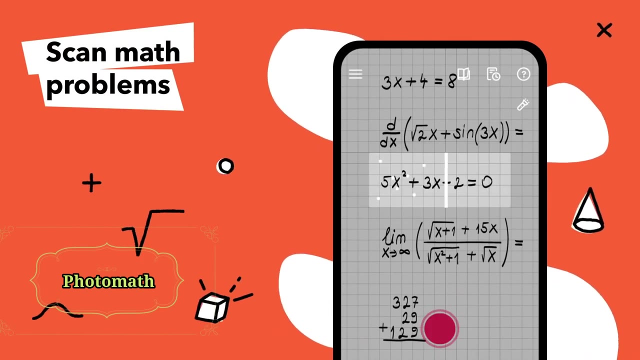 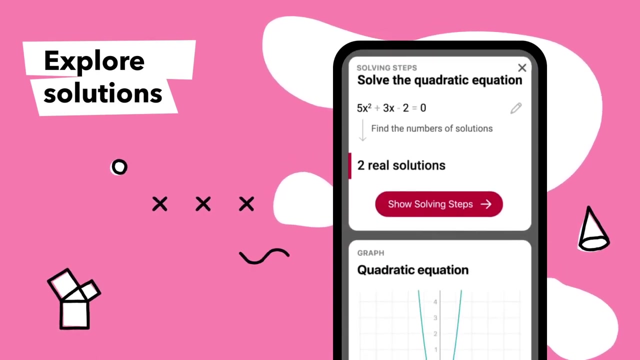 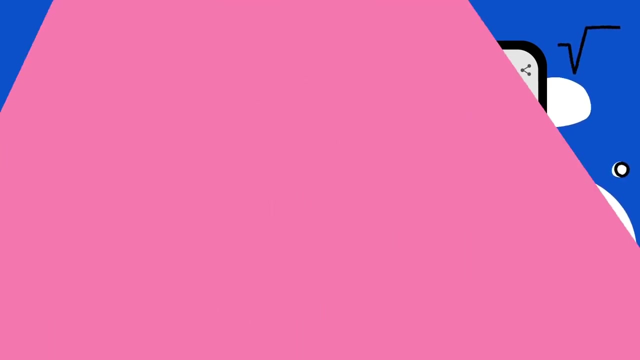 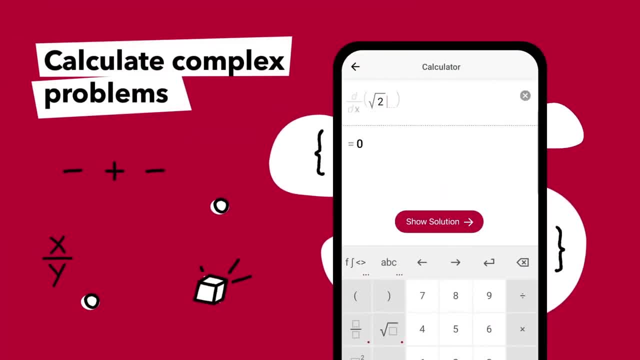 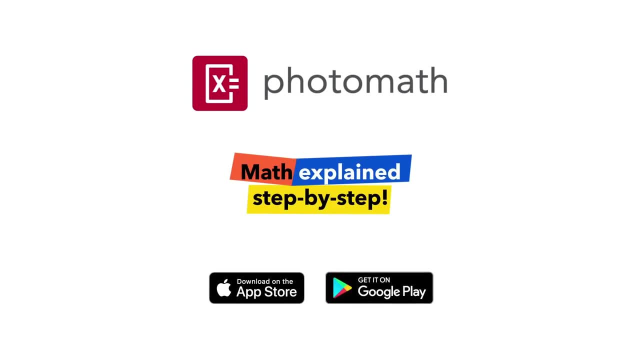 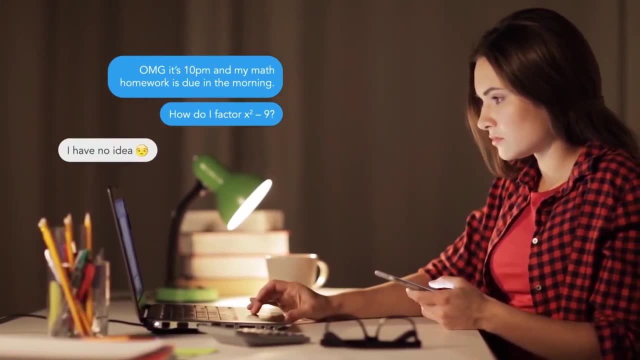 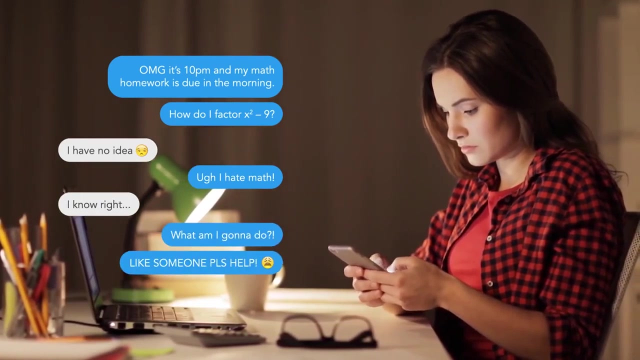 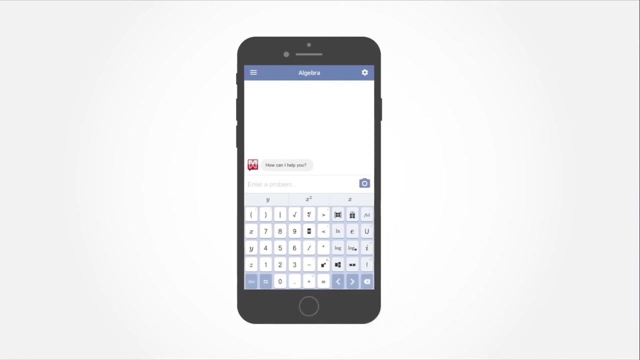 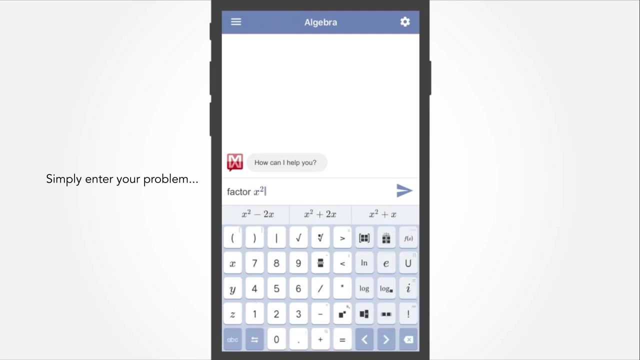 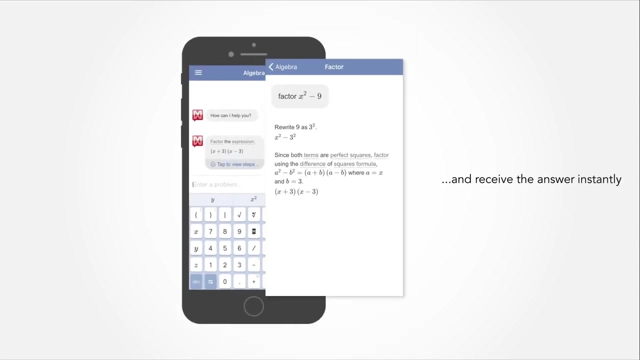 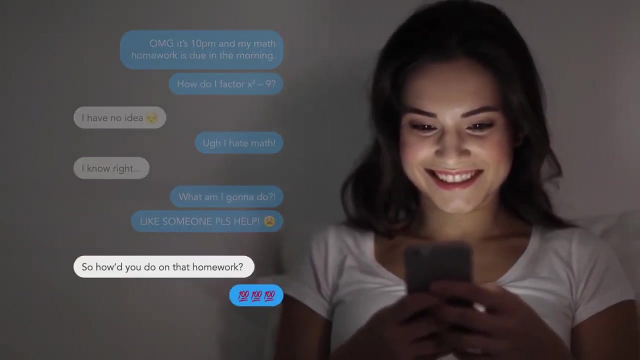 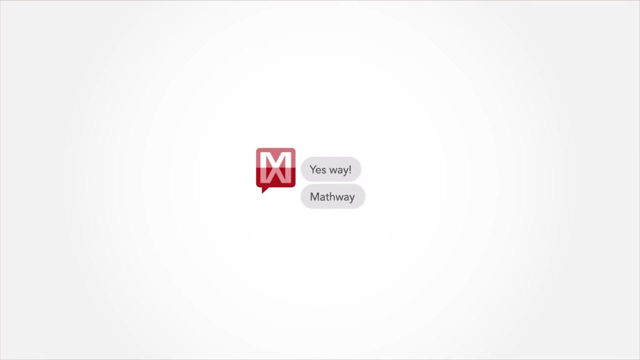 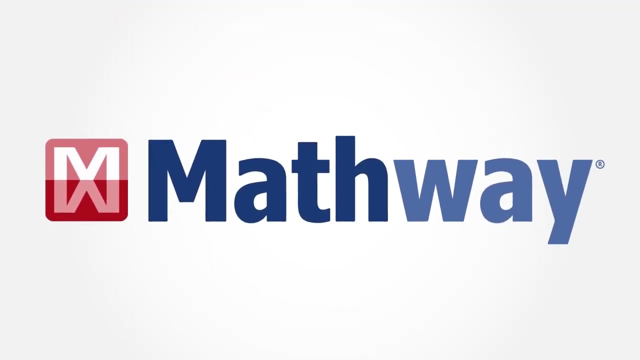 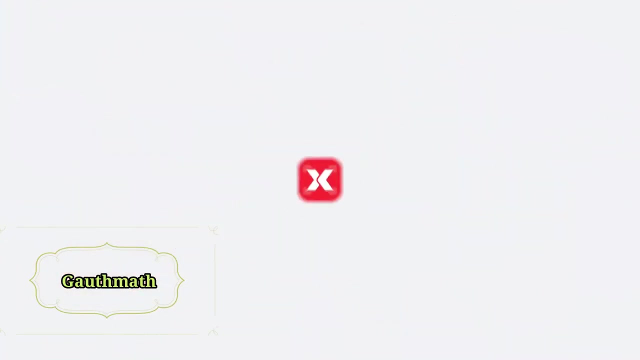 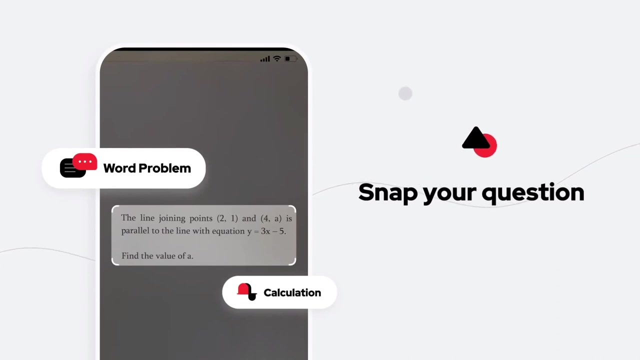 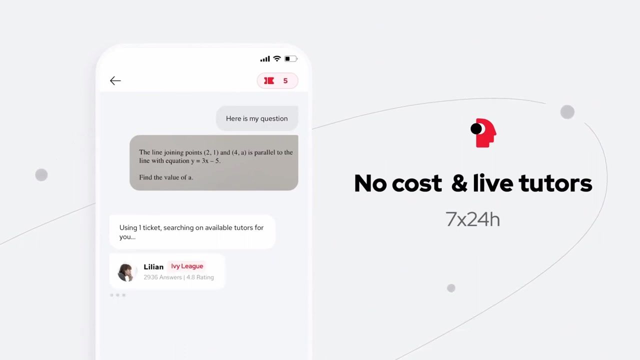 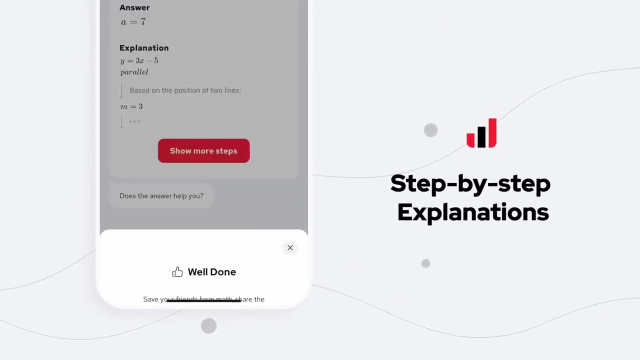 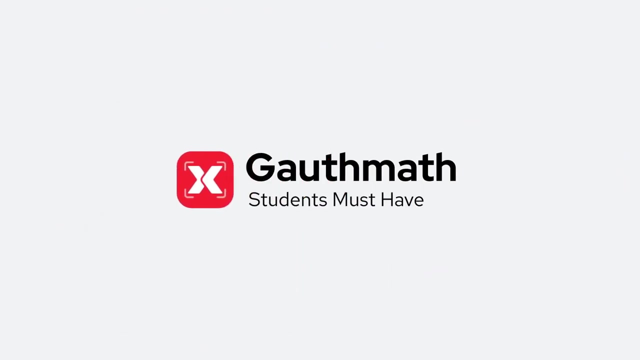 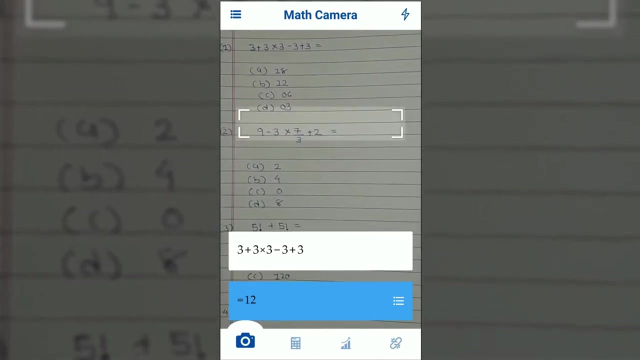 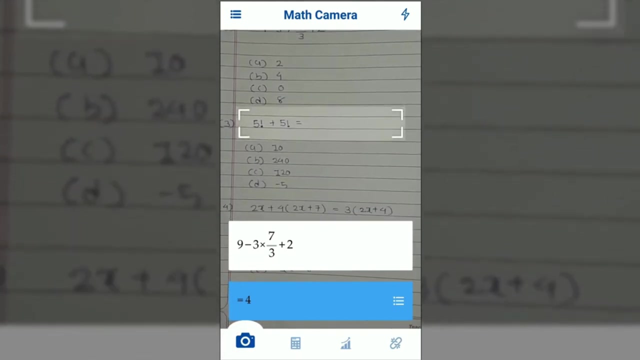 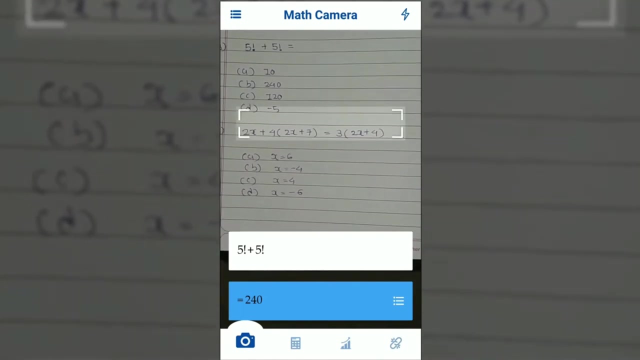 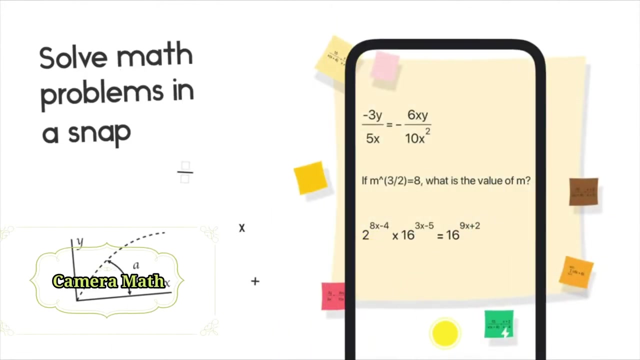